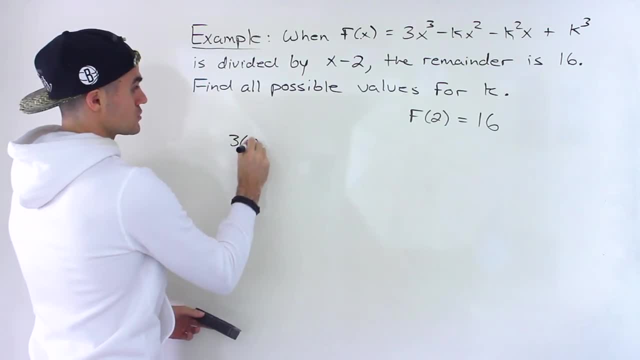 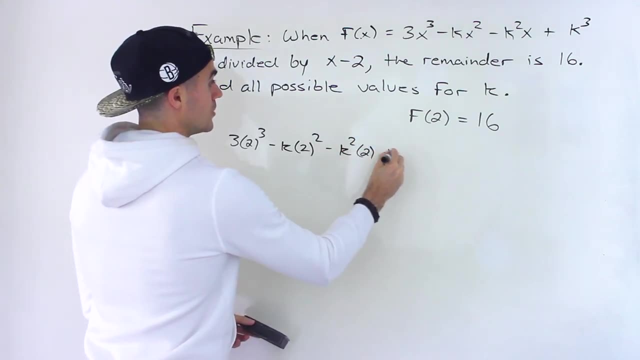 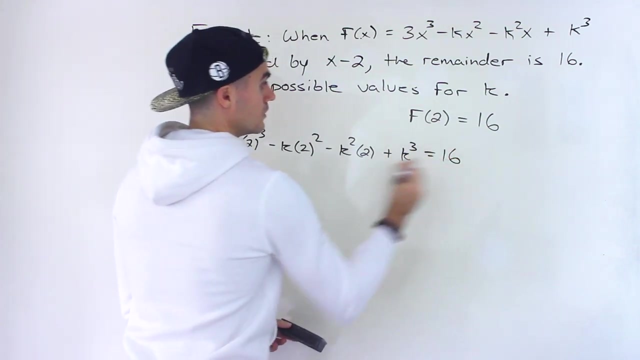 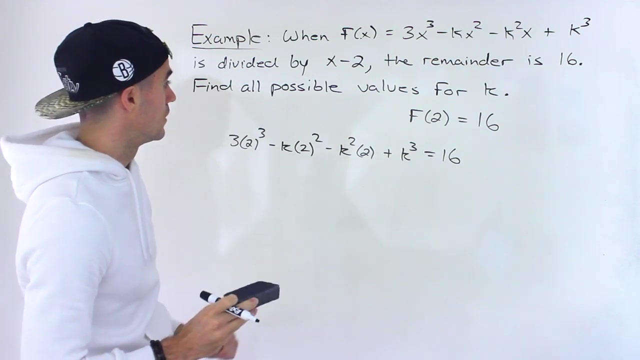 for all the x values. So we'd have 3 times 2 to the power of 3, minus k, 2 to the power of 2, minus k, squared times 2, plus k to the power of 3.. Right, And that's equal to 16.. Right, From here to here. I just plugged in 2 for all the x values. 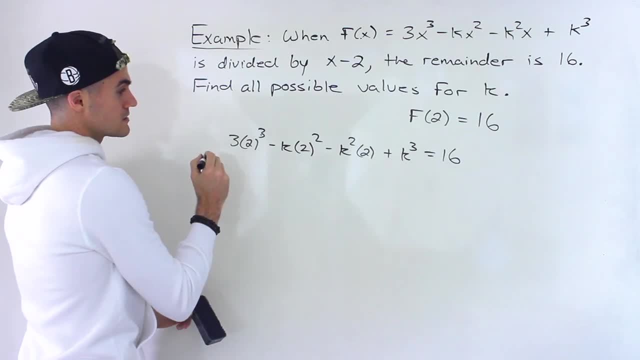 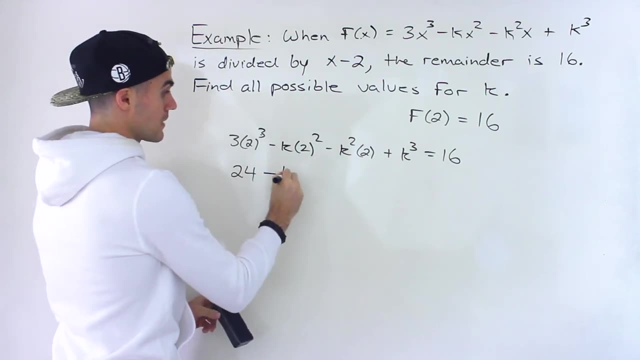 So from here, what would happen? 2 to the power of 3 is 8 times 3 would give us 24.. 2 to the power of 2 is 4 times negative k would give us minus 4k. 2 times negative k, squared would be minus 2k. 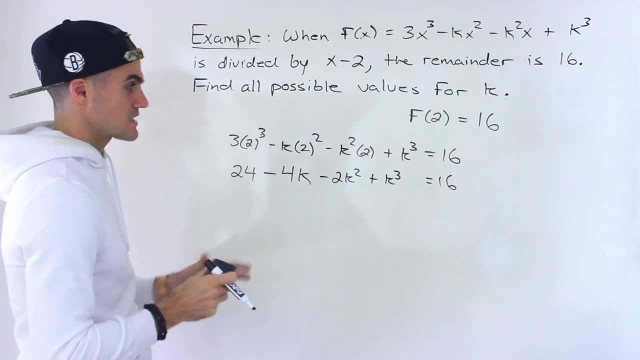 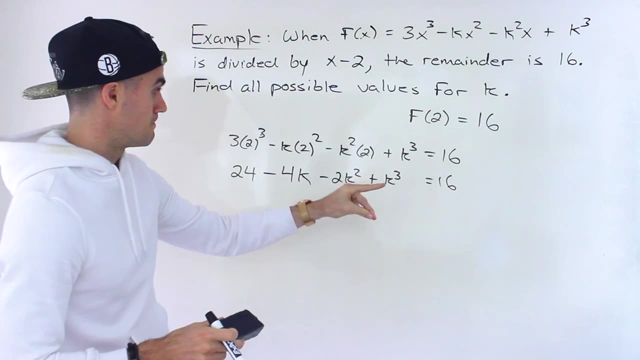 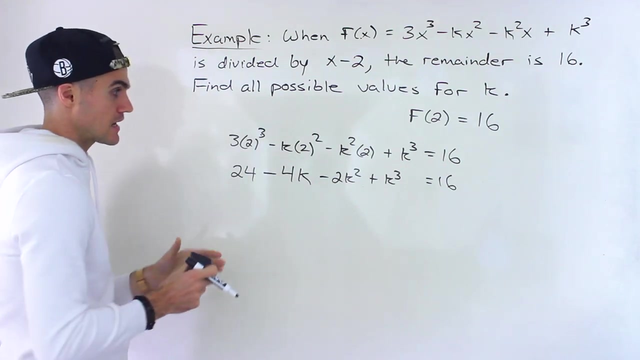 is equal to 16.. And now, notice, we just have a polynomial equation to solve with the variable being k. That's what we're solving for. So what we can do here is we can bring everything to the left side. Let's keep the notice: the leading coefficient is going to be 1,. 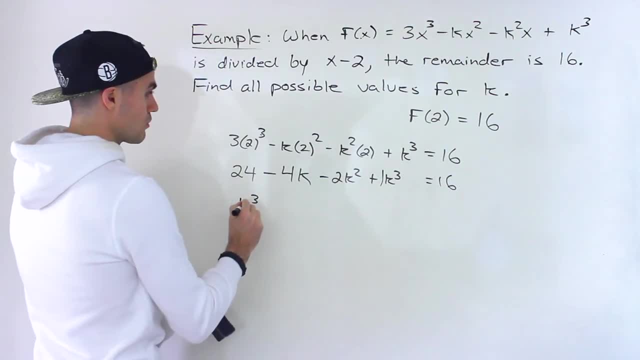 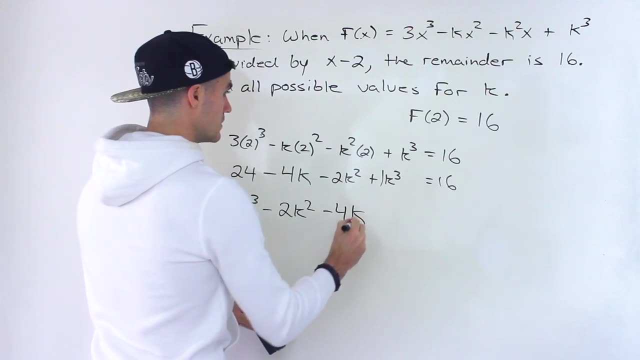 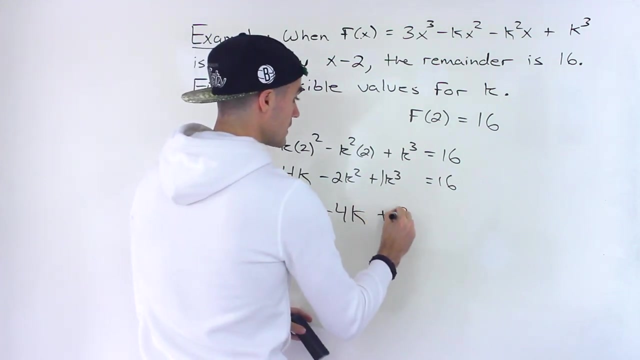 and I want to keep the leading coefficient positive, So I'll put the k to the 3 there. Next would be minus 2k squared Minus 4k, And then bring the 16 over 24. minus 16 would give us positive 8.. 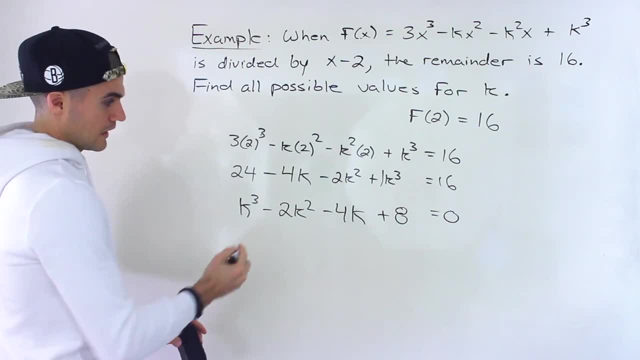 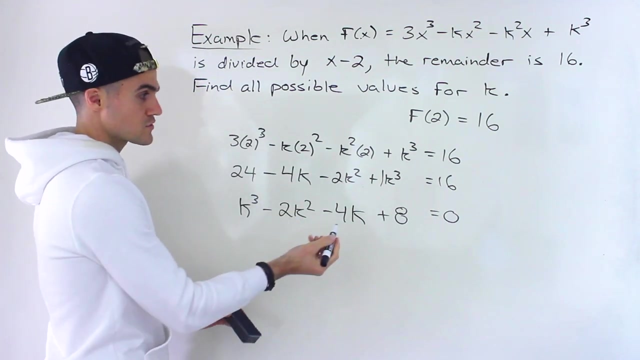 And that's going to equal 0.. And now you just got to solve this here. So this actually factors smoothly And actually luckily we can factor this by grouping. But if you didn't, you can just use the factor theorem, Right, So you could try different values for k. 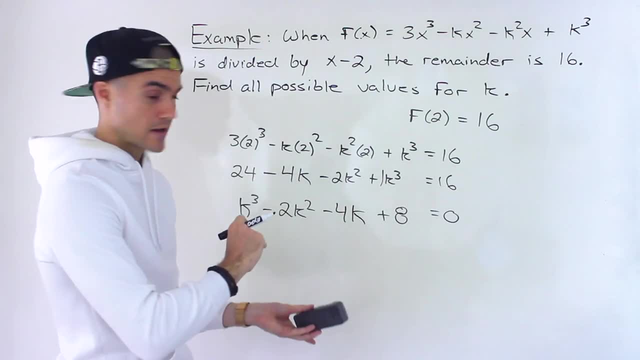 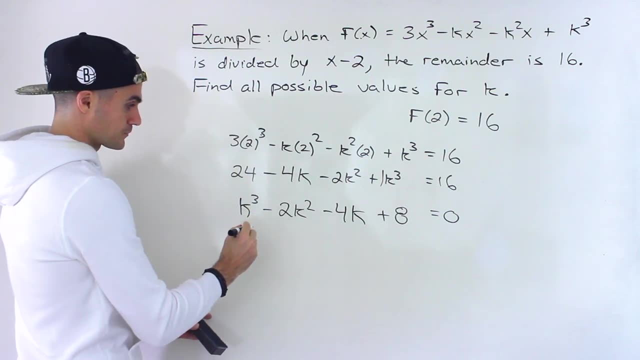 plus and minus 1, plus and minus 2, plus minus 3.. Keep going until you make it equal 0. And then you can do long division. But in this particular case, what's nice is we could take out a k squared from these. 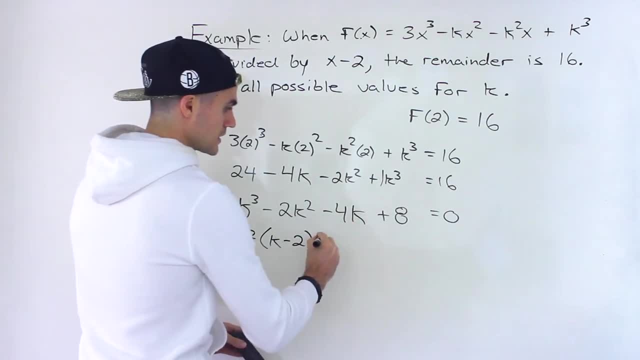 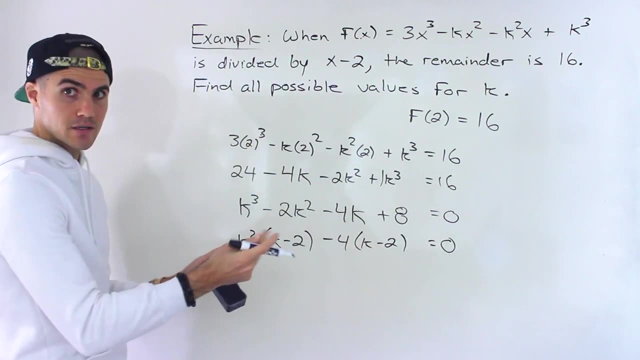 two. So we'd end up with k minus 2.. And then we could take out a negative 4 from these two. We'd end up with k minus 2.. Again, that's not always going to happen, It's not always going to factor. 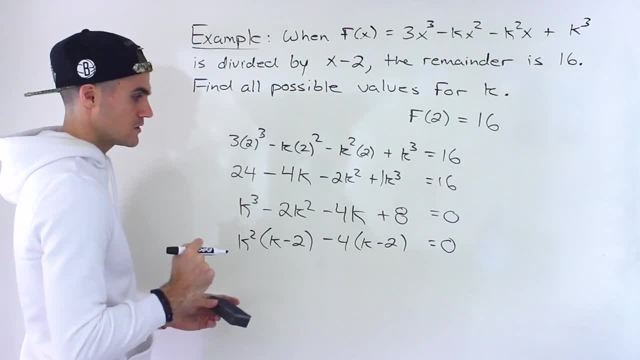 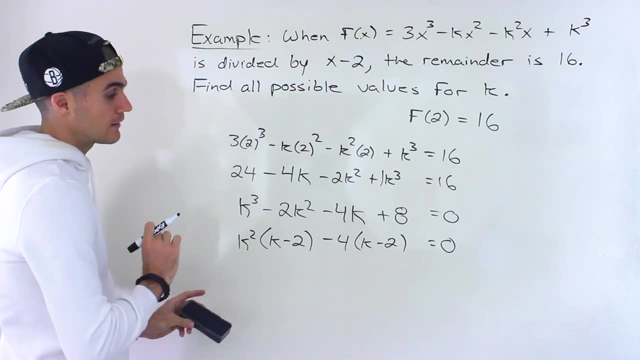 like this. Sometimes you're going to have to use the factor theorem And that takes a little bit more work. But in this particular case it does work with grouping. That's always what I look for. first, Does it factor with grouping, if you get like a cubic polynomial, And then if that doesn't, 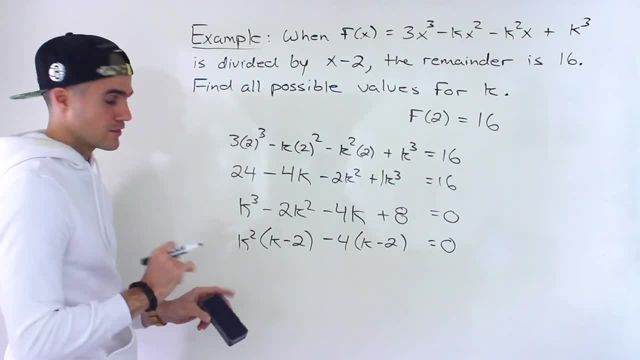 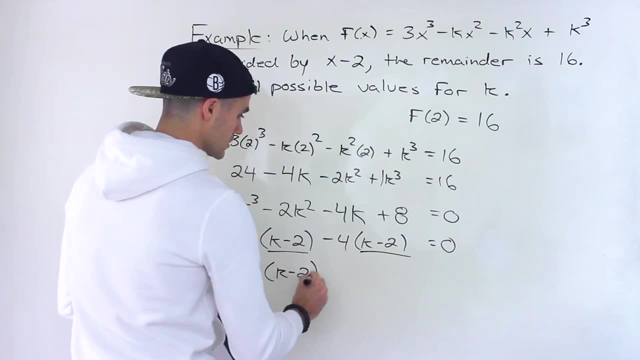 work, then unfortunately you then have to do it the longer way with the factor theorem. But in this case it works because- notice, this bracket, this bracket are the same. We could take that bracket out And we'd be left with k squared minus 4 equals 0.. 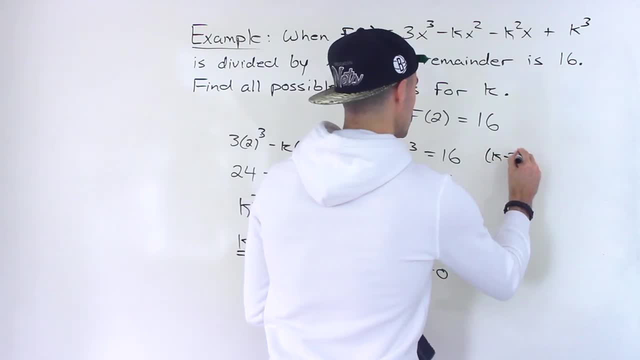 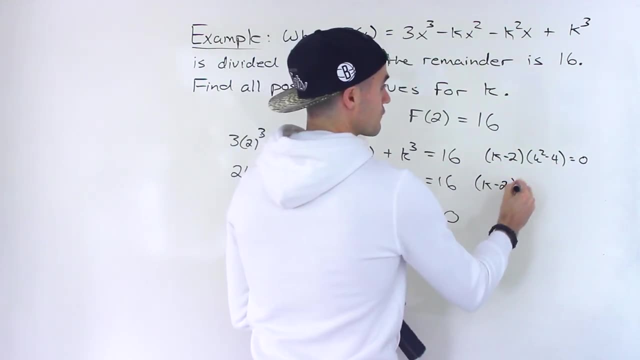 Okay, so then, continuing this over here: k minus 2, k squared minus 4 equals 0.. Notice the k squared minus 4, that factors into k minus 2, k plus 2.. That's a difference of squares, right? And then 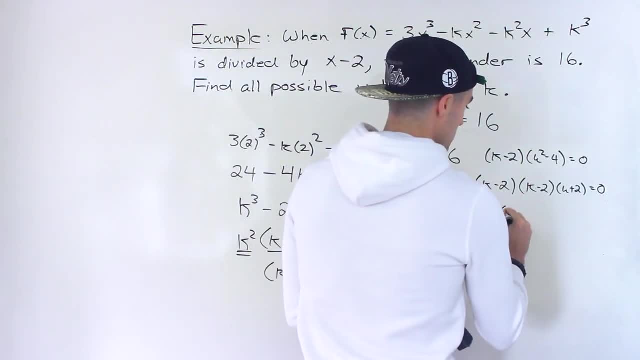 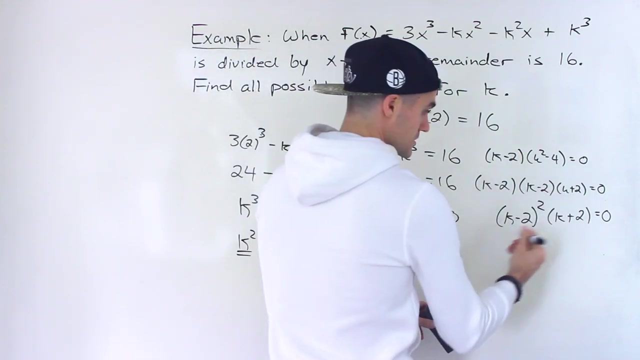 notice this and this same factor, So we can just combine them, make it look nicer. that would be an order of 2. And then we end up with k squared minus 4. And then we end up with that right there, And then from here we know that this has to equal 0. That. 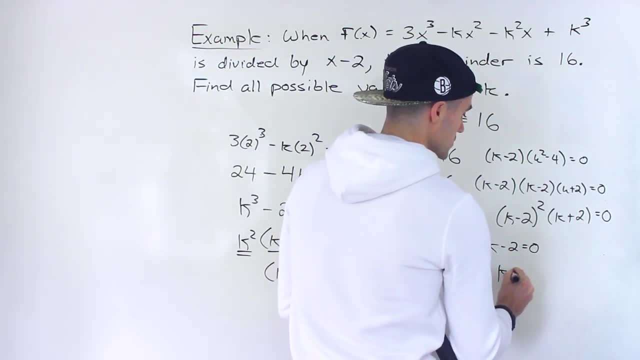 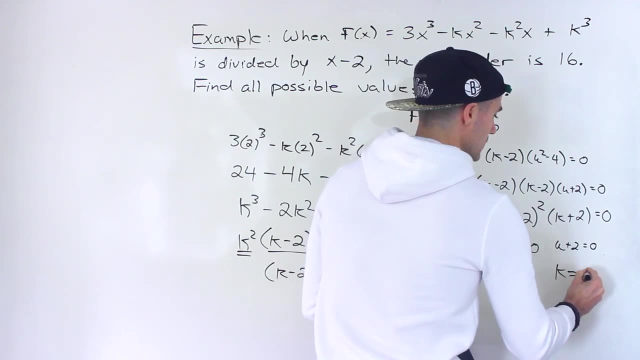 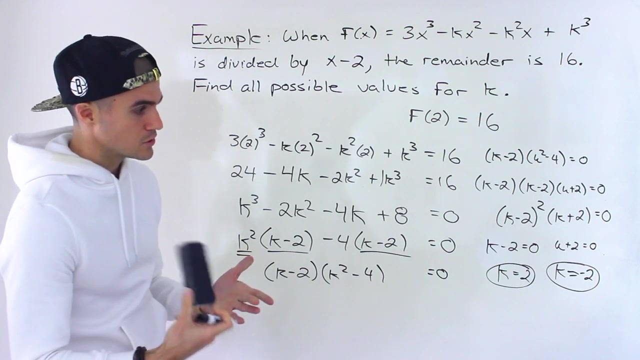 means k minus 2 has to equal 0. So k can be 2.. And then k plus 2 has to equal 0, meaning that k would be negative 2.. So those are the two possible values, right? And then, if you have time, you. 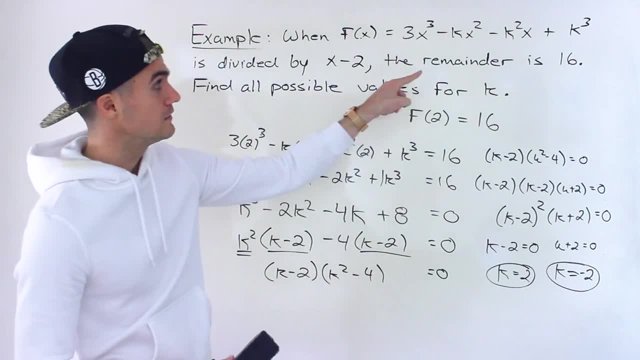 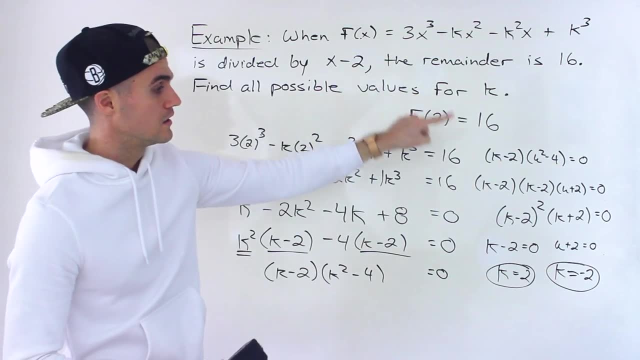 could check your answer. you could plug in 2 for k. you'd get a certain polynomial And then see: does f of 2 equal 16?? You could plug in negative 2 for k. Just be careful with like your signs. 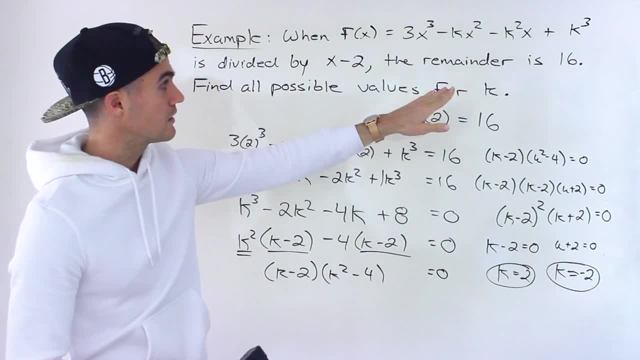 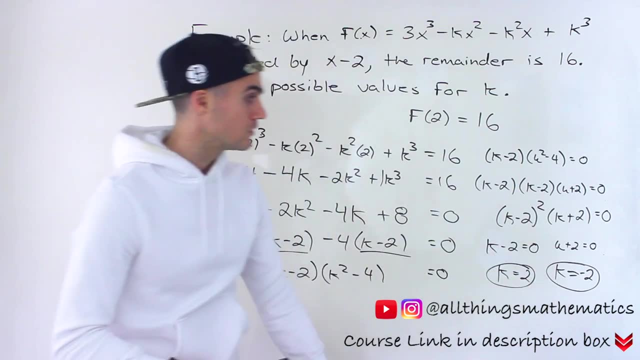 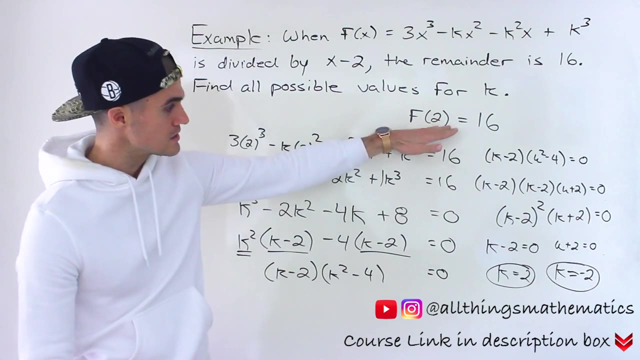 and stuff. Get the polynomial there And then see: does f of 2 equal 16 for that particular polynomial, for the case where we're letting k equal negative 2? And you would see that it does work out right. So make a general statement like this: Just do the algebra. Those are the two k.